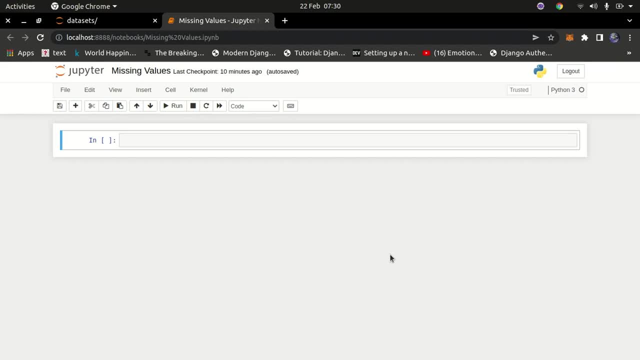 Hello guys, welcome back to my channel. So this video marks the beginning of a new series in my channel. So in this tutorial we are going to cover data cleaning in machine learning or data science. So, as a data scientist or as a person who does machine learning or data science related, 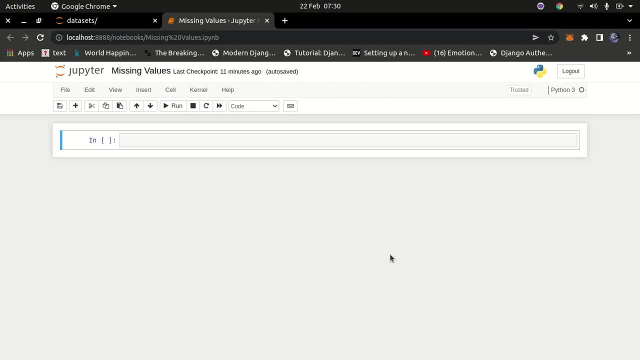 stuff- data analysis or any stuff like that. one of the important things that you'll be dealing with most of the time is data, right? So before you can do anything in machine learning, the first important step you have to do is making sure that your data is clean and you have a good 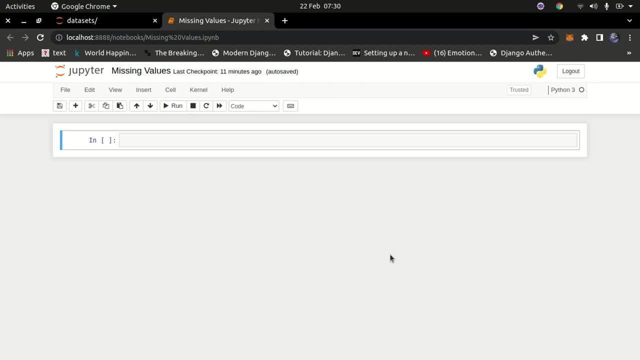 understanding of that data. So in this series you're going to go over and cover how to clean your data properly and use it in your model, because in machine learning, as we usually say, the model is only as good as your data, So your data has to be good for your model to be good. 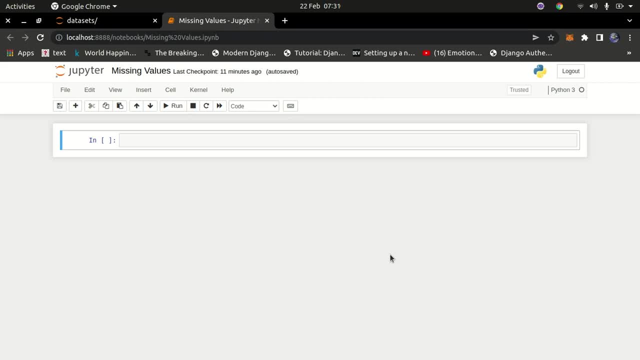 So if you're going to be joining cargo competitions or other stuff, one of the important skills that you need to learn as a data scientist is how to clean your data. If you're working as a data analyst, you need to know how to clean your data. So if you're working as a data analyst, 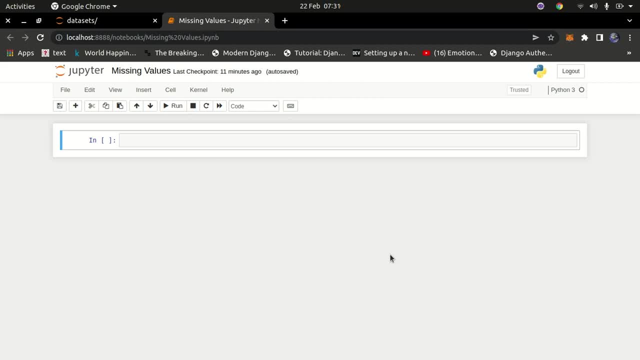 then you need to have a properly cleaned data before working with that data, right? So the different techniques that you're going to learn and that you can use to clean your data. So in this tutorial, we're going to begin with a very simple step of learning of dealing with missing. 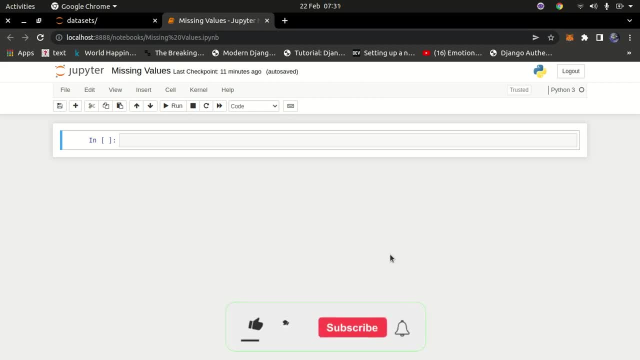 values okay. So if you're new to the channel, please kindly consider subscribing and hit the notification bell so that you can stay updated whenever I upload new videos in this series. So we're going to go over data cleaning and in this tutorial, we're going to go with 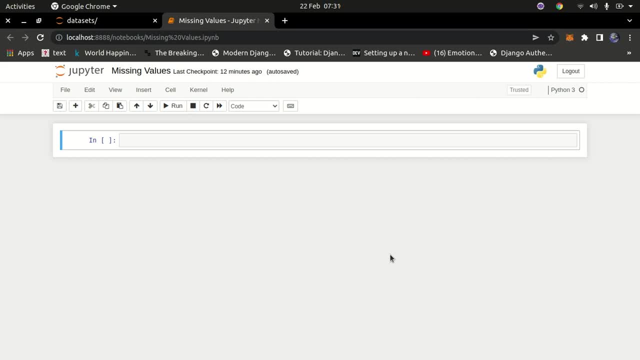 dealing with missing values. So, whenever your data has missing values, how do you go about dealing with that thing? Okay, right, Are you going to impute the values? Are you going to delete the columns and stuff like that, And that's. 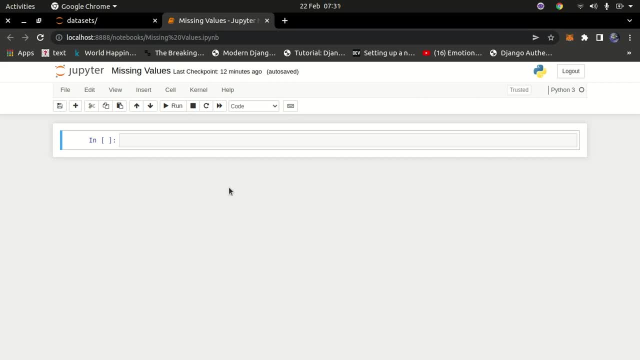 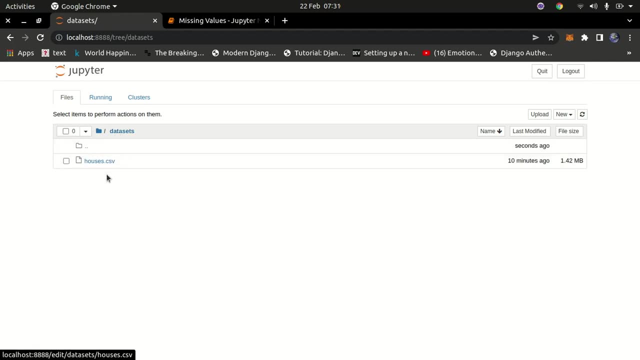 we're going to learn that technique in this video, So let's get started to it. So the first thing you need to do, I have a data set called housescsv. So this housescsv, I'm going to make it available on my GitHub page, and the link is going to be in the description below. So now let's get started. 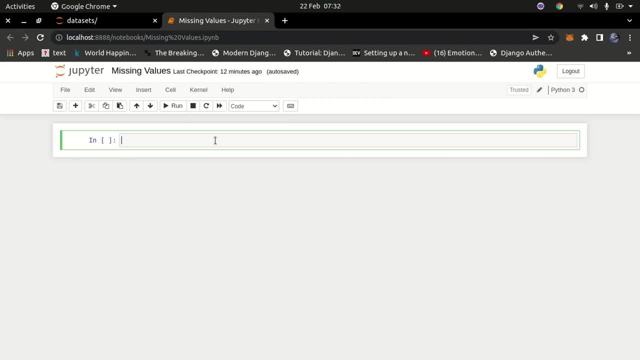 with. let's get started with our today's agenda, which is dealing with a learning how to deal with missing values. So I'm just going to keep a mark down here, just saying dealing with missing values, just like that. So let's begin. So what I'm going to import: 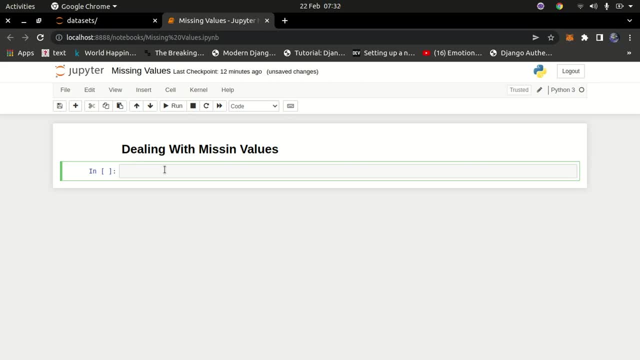 I'm going to import pandas and numpy Again. if you don't know pandas, I have a whole series on pandas on my YouTube page So you can go ahead and check that tutorial out. It's actually a whole series on pandas, So it teaches pandas from the basic until to a bit intermediate level. So 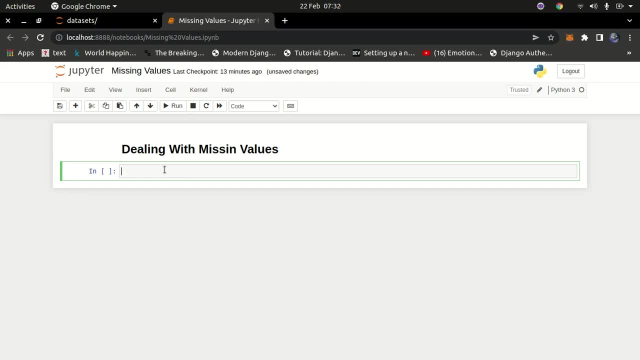 the knowledge of that series will be completely sufficient for this course. Okay, so I'm going to go ahead and import pandas as PD. I'm also going to go ahead and import numpy as MP, just like this. So I have went ahead and imported pandas and numpy. So once I have those two imported, 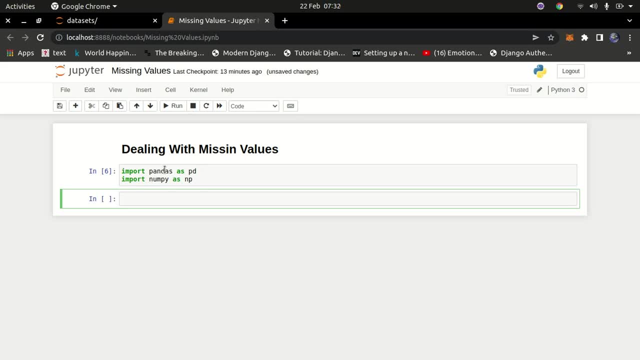 you can begin. So the first thing to do whenever you have data is, first of all, you have to know how your data looks like. Just open up your CSV file and then just see how your data looks like, what information it provides you and how you can use the information you have to solve. 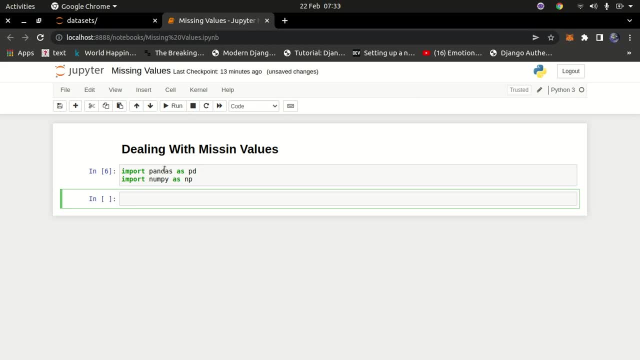 the task that you're given. So it's very important that we look at our data. So let's go, let me just write a markdown here: How. let me just say how. how does the data look like? Okay, So it's very important that you know how your data looks like, because you know what features. 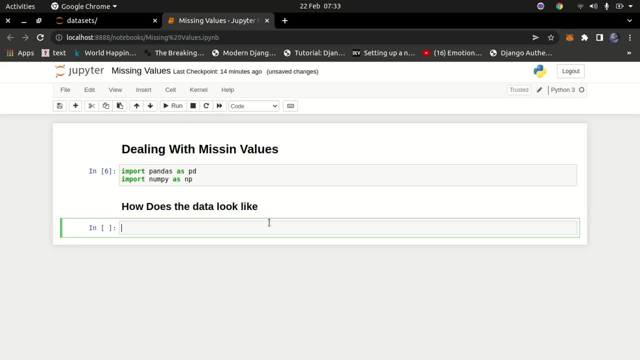 you have how to use those features to achieve the important task that you want to do. So, first of all, what I'm going to do, I'm going to first read that into a data frame, So I'm going to say pd dot, read underscore CSV, And in here I'm going to provide the path to this, which is in: 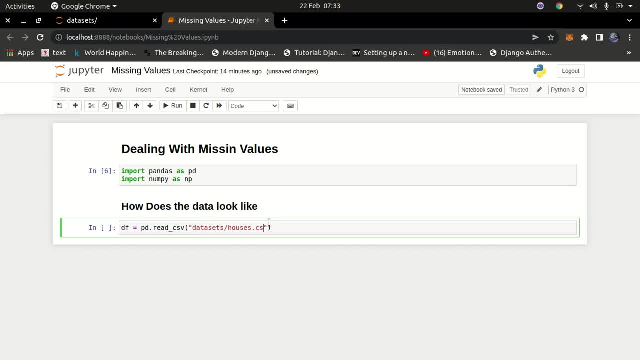 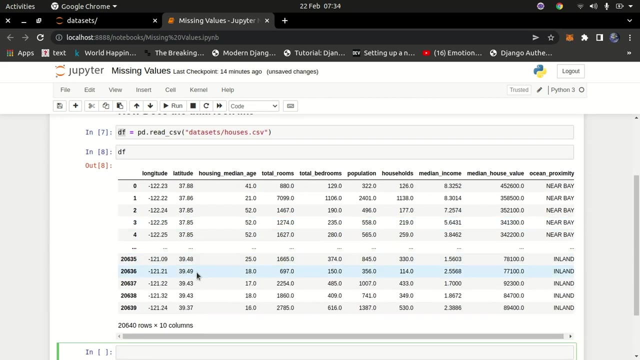 data sets folder for slash: housescsv. Okay, and I'm going to run that and this is going to read for me my CSV file into my data frame. okay, variable right here. So I can just do data frame right like this. You can see, I have all this, all these features right here. So the what you can you. 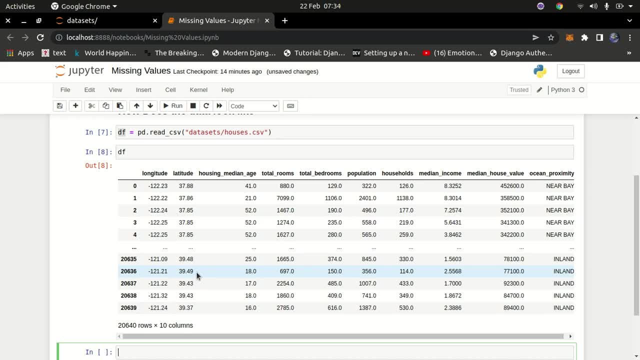 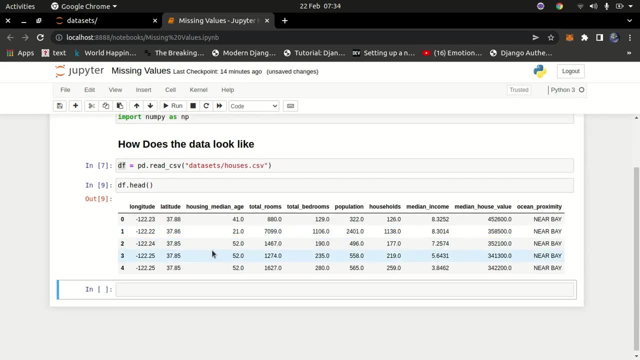 cannot look at the whole data, and most of the data is just too much to look at all of it, So I'm just going to look at the head, the first five rows. What about the first five rows? Yeah, So you can see. there's a data that we have and you can see. 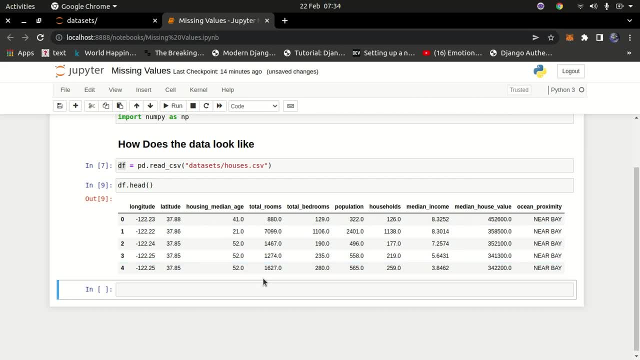 each of those feature names that we have. So we have a column, we have the column of longitude, latitude, house, medium, age, the total and the total number of rooms, and all this. So it is a data set about houses. Okay, So you're going to use this data set to deal with how to 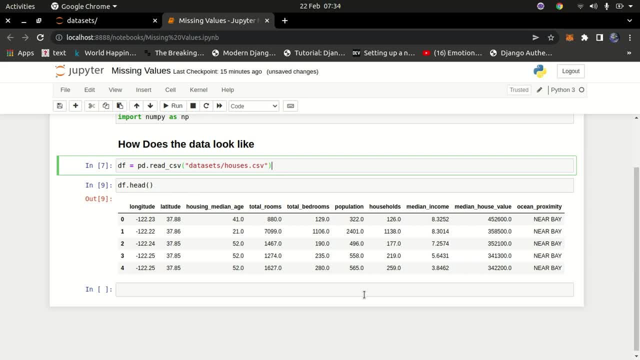 learn how to deal with missing values. So now that you have been able to look at our data set and we know what the data is all about, right in this case. in most cases, you have more information. maybe there'll be a documentation or the data set or something similar to that, But in this case, this. 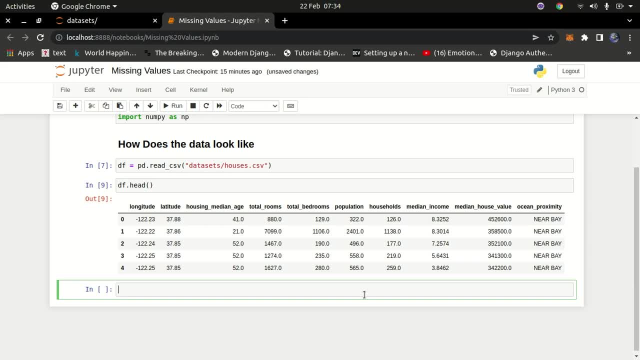 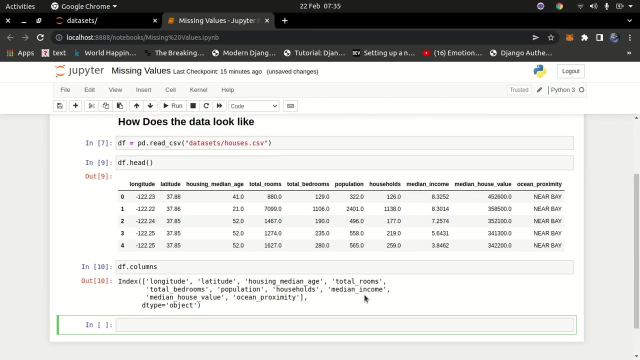 data set. you have in this what you're going to work with, And you just look at the end of data that we have in the number of features that we have. So let's do a DF dot. We can even count the number of columns. I think you just say columns. So this is going to return to us the number of. 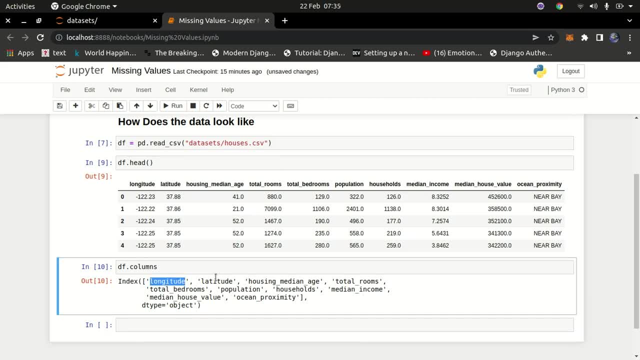 columns that we have. So you can see we have all these columns. we have the longitude. you can also do, we can also count this. if you want that. you can do the length of it And you can see how many total number of columns. 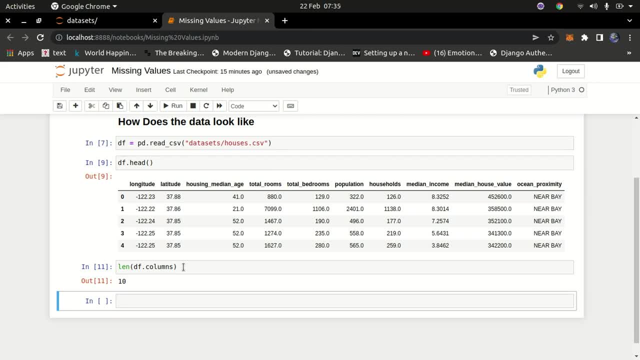 we also have 10 different columns in our data sets, So you can- you can also print out all of these columns, which are all of them here. you don't need to print them out, actually. So we have 10 different columns of our in our data set, So now we have a hum. you can check the shape of the data. 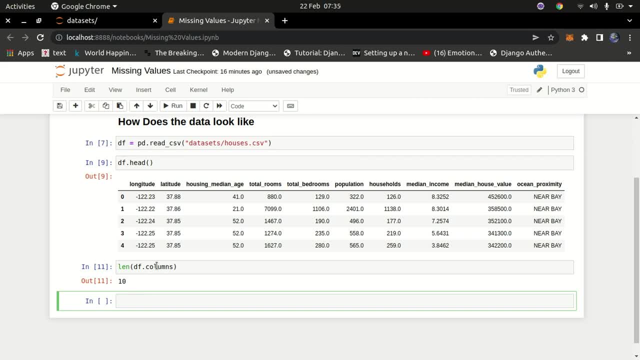 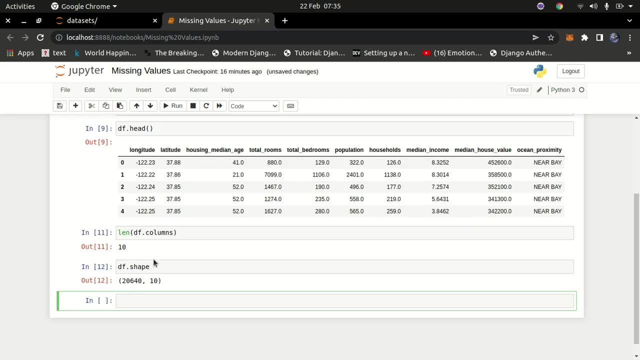 set to know how many rows. and now we are dealing with we know how many columns, which is 10 columns. So let's do DF dot shape. if you give a shape, it ready that same information, So you can see we have shape it. 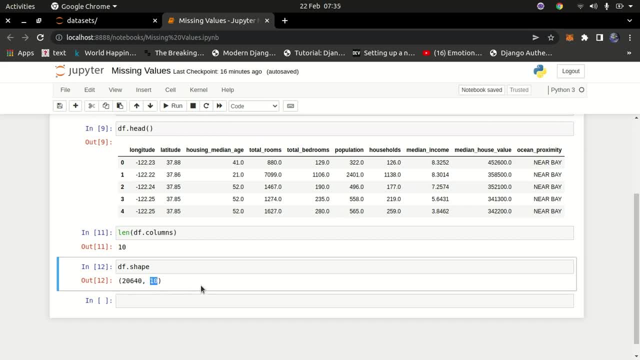 answered the number of rows and number of columns. So we have 220, 20,640 rows and we have 10 different columns, which is the same value as this one. So now we have a brief description of our data set, right, So we can even do DF, dot describe, And that should give us more information. So this: 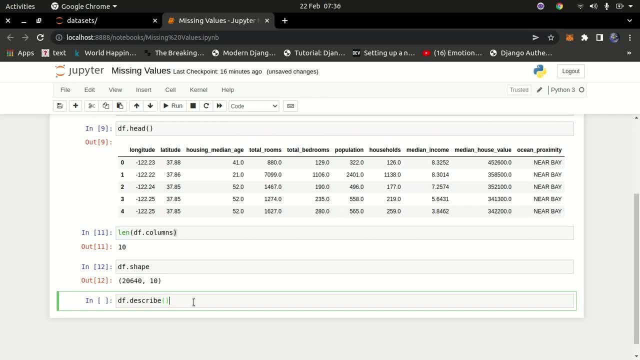 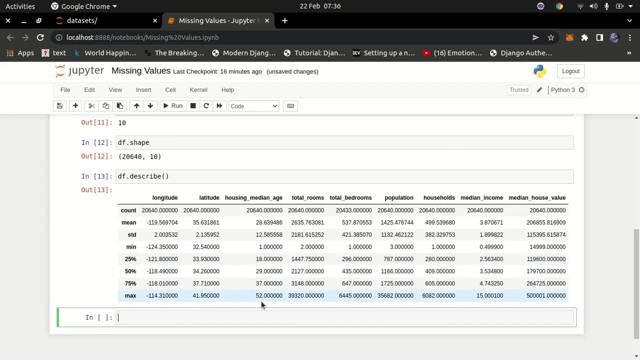 idea to describe, describe, just like this. And if you run this function, you can even get more information About the marks, the mean, the standard deviations and other stuff like that. And means, the sand deviation, the, the 50th percentile and other details like that. So we have all that detail. 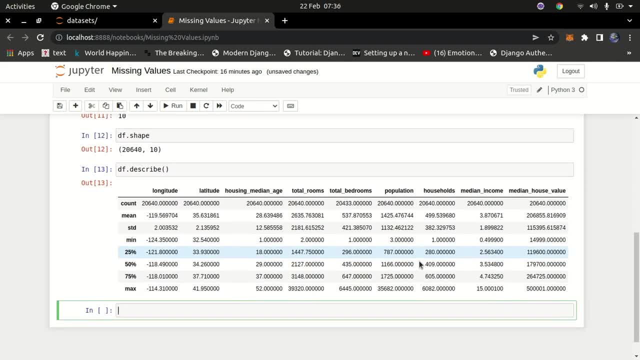 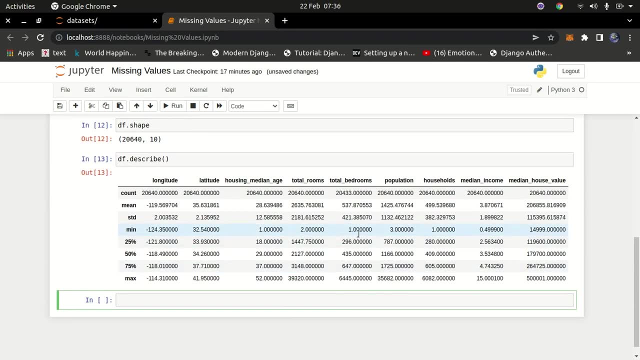 here. So this is a short description of our data set. So now we know we have a data set having over 20,000 columns and 10 rows And these are the different: the mean, the max and values of each individual column. So we just have a very quick description of our data set. 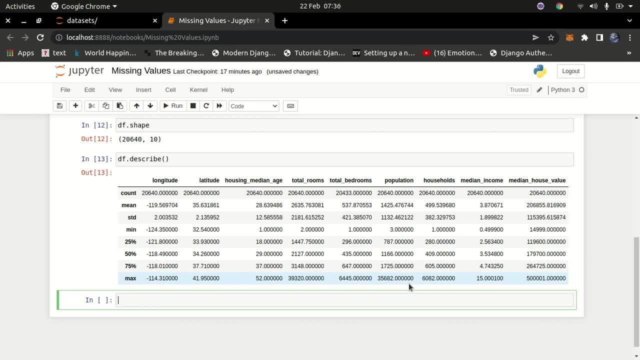 Yeah, Now, in this case, most of the time, your data set may have missing values, right? So we want to check how many missing values are in our column, because that's the main aim of this tutorial: to know about missing values. So let's check, Let's check how, let's say how many, how many missing values do we? 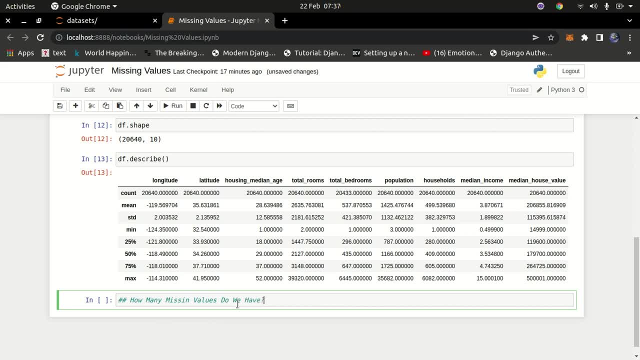 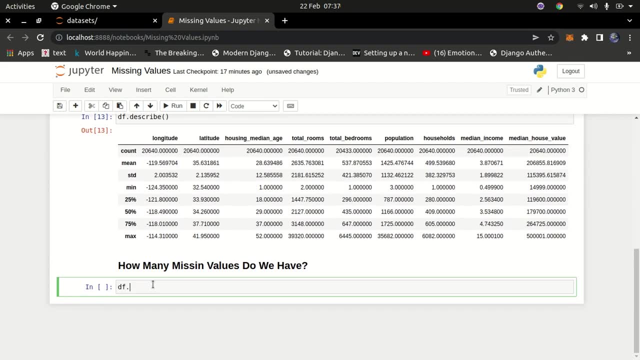 have. How many missing values do we have? So let's check that up, That's argument, Let's see. let's answer that question. so we want to know how many missing values are inside of this data set. so we can just do df, dot is na. if you do this, it's going to return to us this right. it's going to return to. 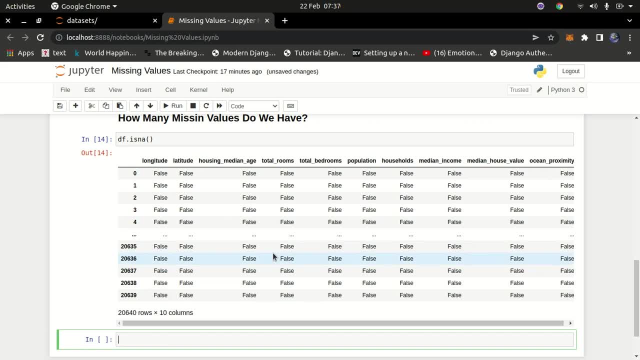 us this data from rotating true and false. okay, so whenever it is false means that it's not missing. whenever it's true, that means it's missing. now it's very difficult. you can go ahead and inspect all of this, so the best you can do just do that sum, and this is going to return to us the sum of. 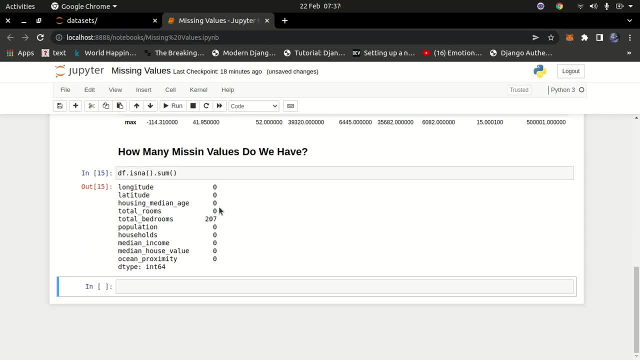 each column. so you can see this, the missing values in each individual column. for the longitude column, you have zero. for the latitude: zero. house age, median age: you have zero. the number of rooms: you have zero. the number of bedrooms: you have 207, 207 missing values. so you can see that's. that's the. 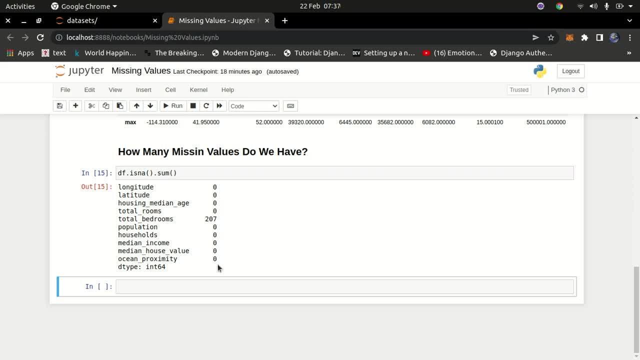 the column containing most of the missing value, and all the other ones have no missing values. so let's go ahead and see how we can deal with that. so we can deal with that very simply. the first thing we want to check is we want to know the percentage of the data that is missing. so 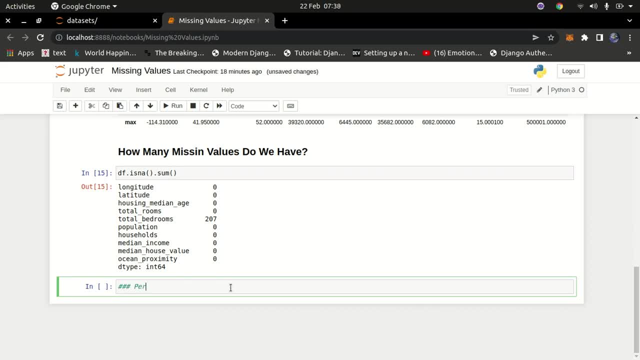 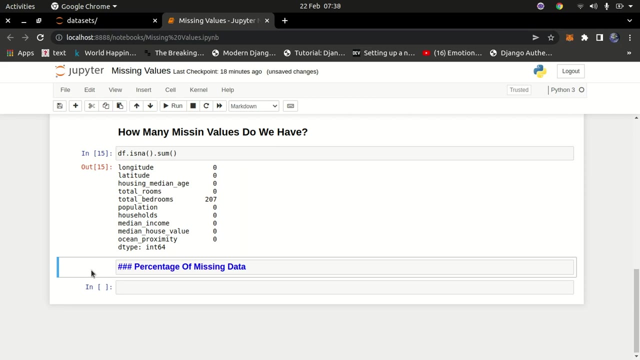 let's go ahead and actually check that. so i'm just going to put a mark down here: uh, percentage, percentage of uh missing data. so i want to find the percentage of the missing data. so let me just make this one to be a markdown cell. uh, just press, just click on your on your cell, on. 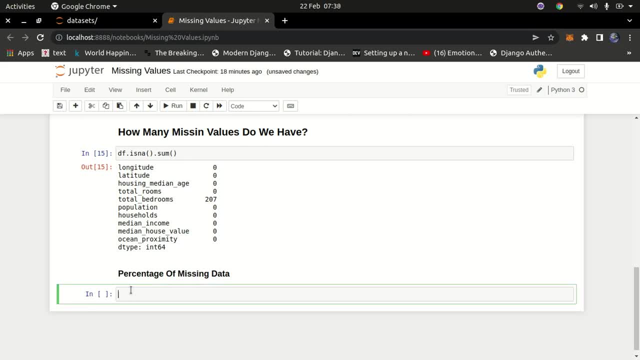 this side and then press m on your keyboard. yeah, that will make it a markdown cell. so once we have that done, uh, let's go ahead and actually check how total total cells that we have. so to do that, no, no mistake, there are the total cells that we have. 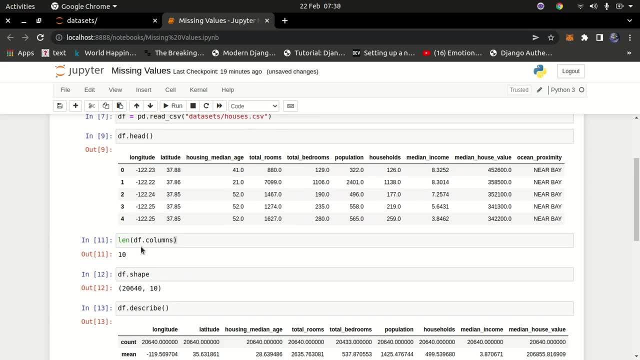 we're going to take the number of rows, right number of rows in our, in our data set, minus the number of columns. in each number of rows, there's a number of columns that return to us the number of cells that we have in our data set. so to do that, i'm just going to say total, uh, total, underscore. 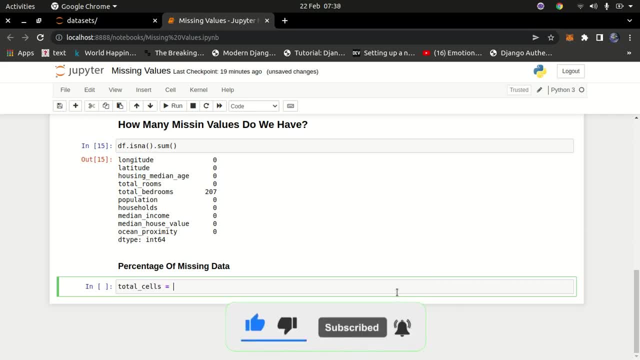 cells, uh, sort of cells, and this is going to be: uh, i'm going to say np, dot product. i'm going to simply just pass in uh, df, that ship. so it's going to multiply if i do, if i go back here, you can see dfshp. 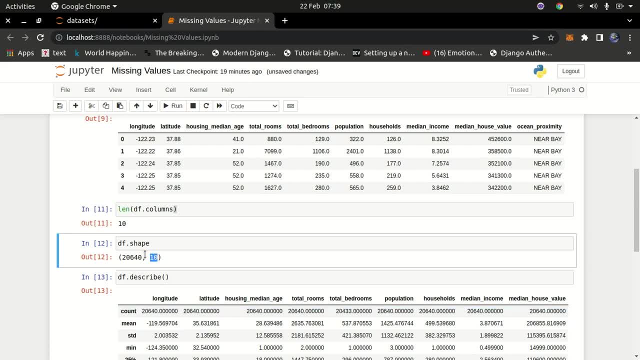 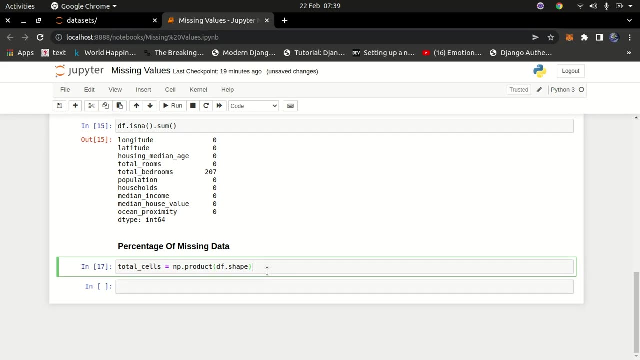 is going to return to us this tuple, right? so it's going to multiply these two values and it's going to give us the response. so it's going to be around. uh, let me see, it's going to be around. uh to 206 000, uh. 40, right, something like that. so if i just multiply this and i can also go ahead and print. 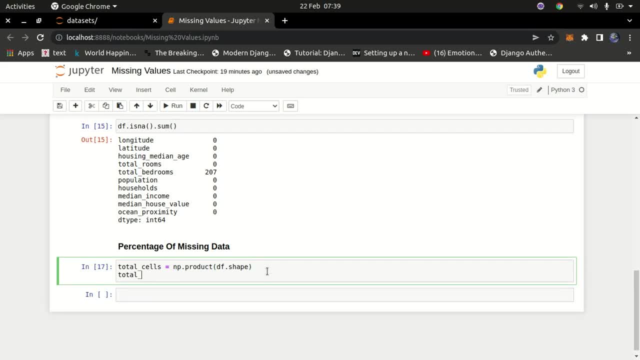 this also just uh do total, uh underscore cells. so if i run that you can see we have uh 200 and uh 200 to 206 thousand four hundred cells. right, so now you can see this and the two number of cells that we have in our in in our data set. 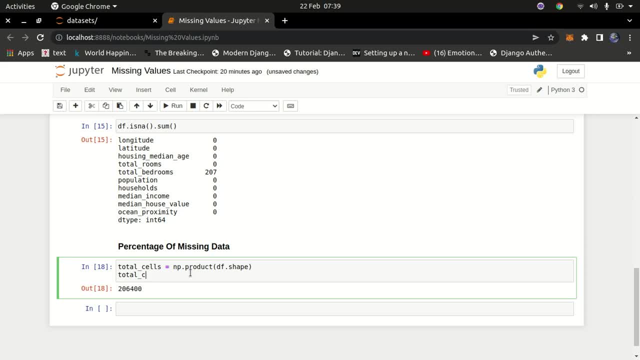 now we want to calculate the number of missing, the total number of missing uh missing values. so i want to say missing, total missing uh, missing underscore uh values. let me just create it on missing values and this is going to be the following: it's going to be: uh. it's going to be the following. so what we're going to do, we're going to: 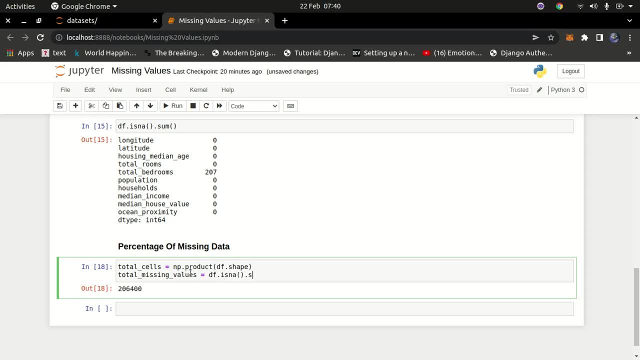 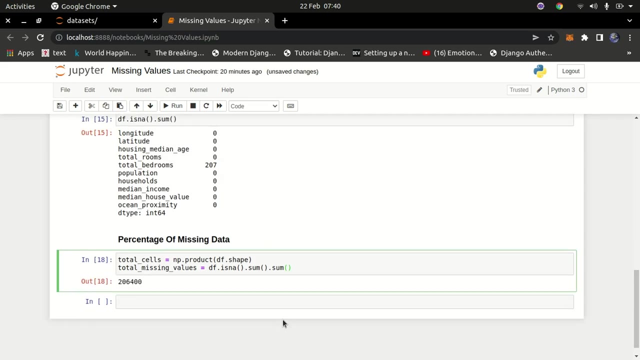 do a df dot is an a dot sum. it's going to return to us the total number of of missing values. okay, we have that value. what you can simply do: uh, let me just uh do that sum here again, because if you do just this, it's going to return to us this value. now we want to find the sum of this value, so if i 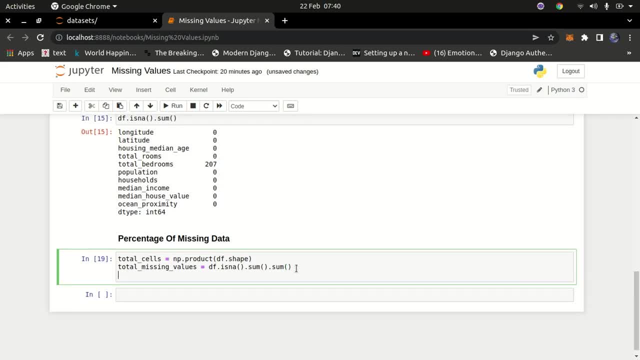 run it. yeah, now everything should be fine. so what i want to do is to find the percentage of the missing data, so i can say percentage of underscore missing data, and this is going to be very simple to do, so i'm going to simply going to do the following. so i'm going to simply take the total. 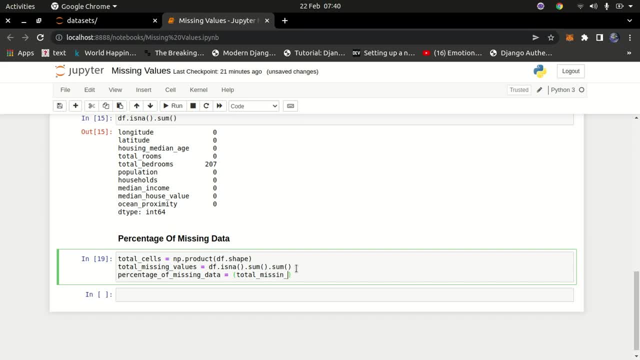 the total underscore. missing underscore values over the total cells. right, total underscore cells. uh, then we're going to multiply this by 100 to get the percentage, and i'm going to do percent, total percentage. i can just go ahead and copy this and then simply paste it here and then run the code. 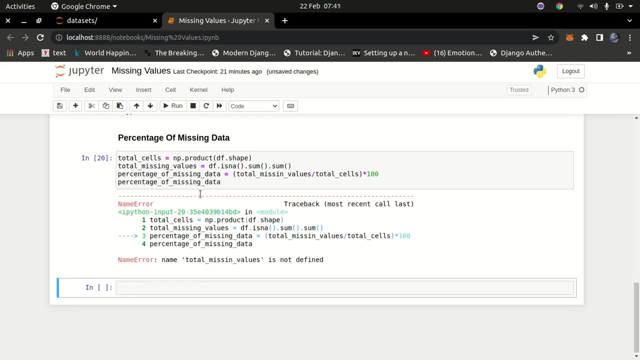 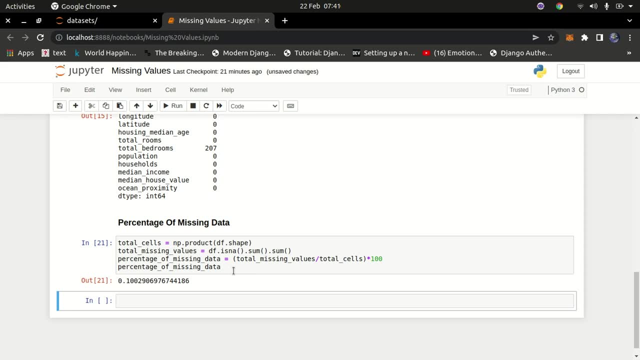 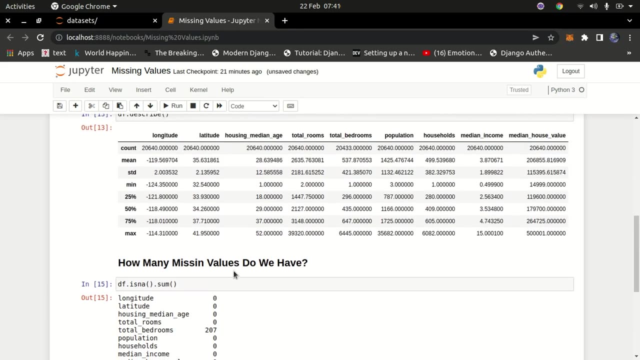 again. so i got an error here. so it says total missing. uh, okay, this is total missing. so let me get the spelling right so you can see we have a zero point. uh, one zero, zero, zero, two nine. so just a little percent of our data is missing. so this is it. is quite, very, very clean, okay, so in in case, if you're working. 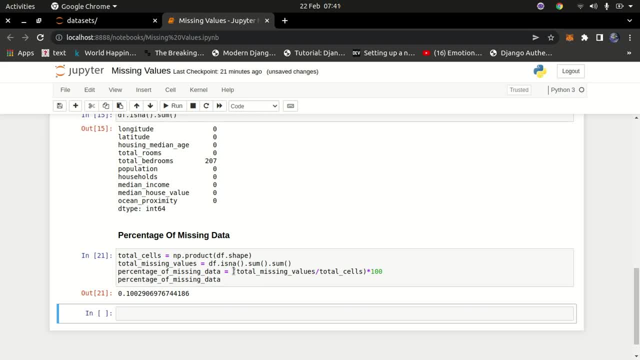 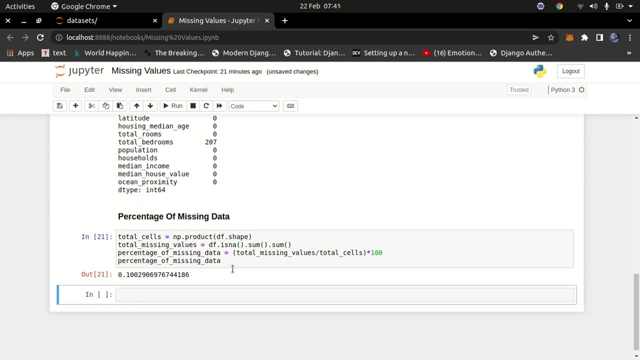 with other data set, you might have ten percent missing values, at that twenty percent. so it can be really uh difficult if you don't clean your data set and that to make your model to be really poor, okay. and if you don't, if you have any values like this: 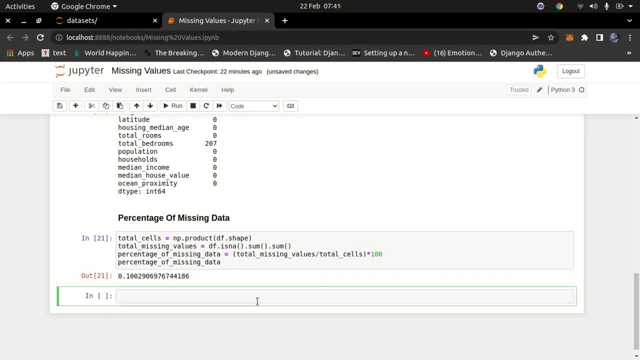 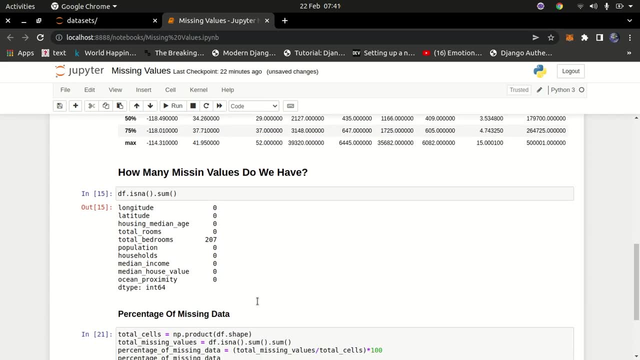 you actually get an error when, uh fitting, trying to fit a model. so what you're going to do is find out why we have missing values. okay, one of the important questions you have to ask ask yourself: after identifying missing values, you have to ask yourself: why do, why do these missing values exist? 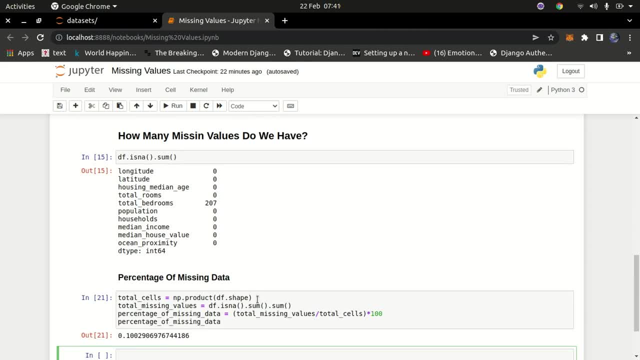 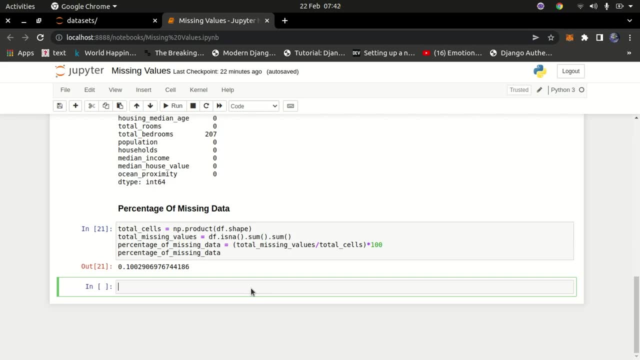 so missing values can exist for various reasons. the first one is that the missing values are not recorded or they don't exist. so let's say: let's say that they are not recorded, so let's say that in this case we have a house data set right, so you can see that the most of the missing values 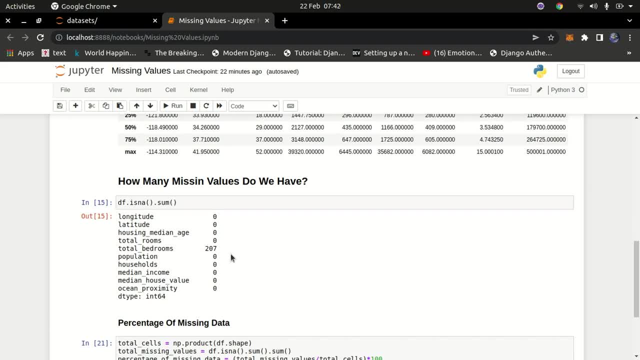 is inside of the total bedrooms column, so that the total bedrooms column is inside of the total bedrooms column, so that the the bedroom not exists, or it was simply not recorded. so in this case it looks like it wasn't recorded right, because a house probably has a bedroom right. 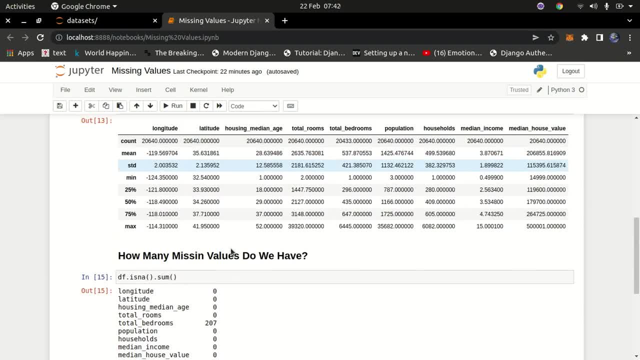 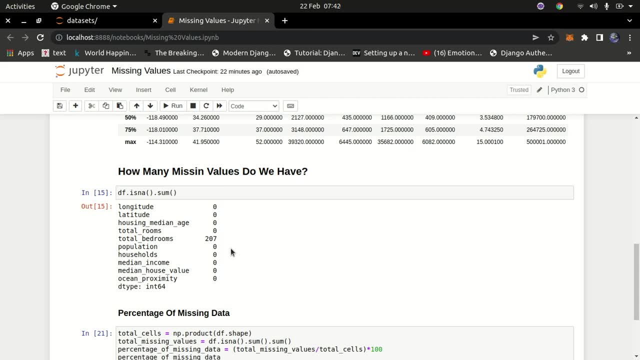 because, besides this, residential uh data, residential houses data, right. so in each house, each house has a bedroom. so what we are we can say in here is that that data was not uh, was not recorded. okay, we can say that the bedroom don't exist, so the bedrooms are simply not. 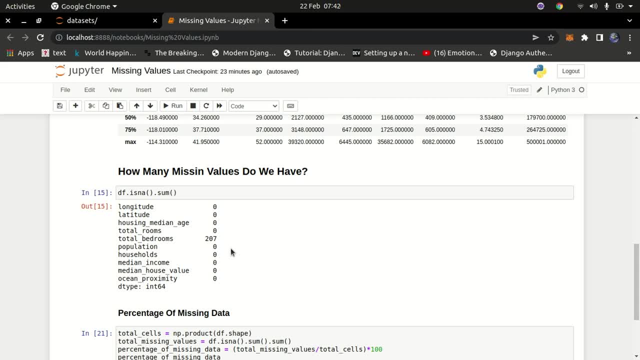 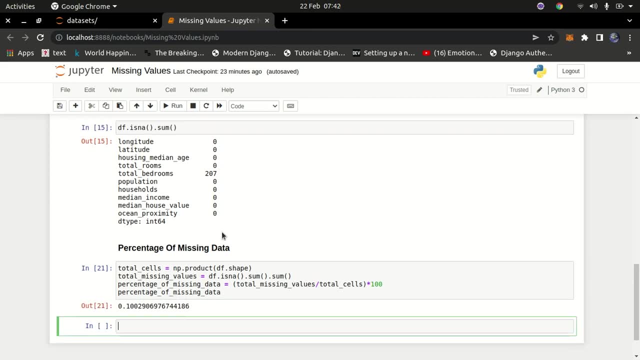 recorded. so in this case case, if you have a data set you can do, you can go to online, do some quick google search, read the documentation of data set and try to find out more information from the people who collected a data set or about resources about that data set, so it can get information about why missing values exist. 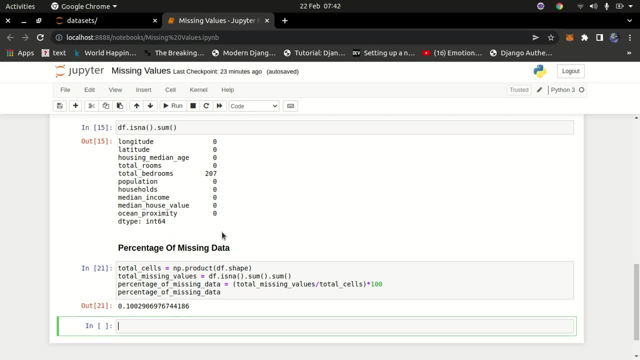 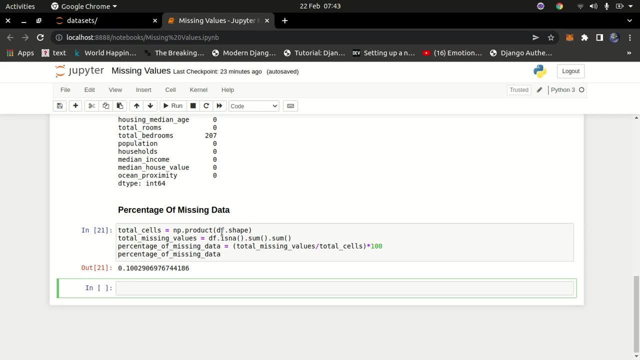 either they are not recorded or they simply don't exist. okay, in this case, it looks like they are simply not recorded, so, um, so, yeah, one way we can fix, fix this- missing values- is by using a method known as imputation, and we're going to cover imputation later on. so there are many libraries. 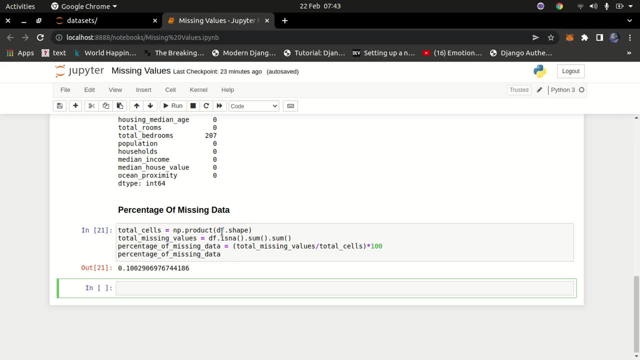 that you can use to deal with imputations in python, and we'll look at that later on in the future. uh, but um, one we can do. one way we can solve this error of having missing values is the first. the first method is by dropping these missing values. we can just simply go. 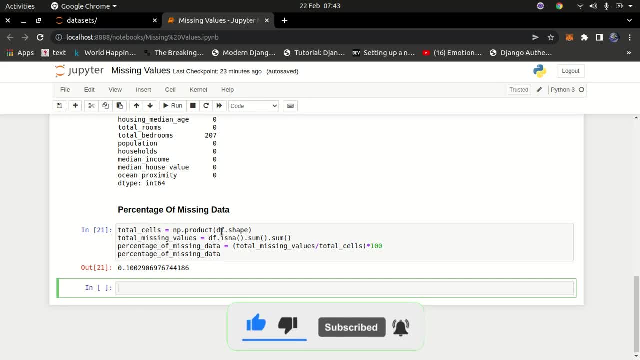 ahead and do a df to drop and that is going to get rid of all the missing values. so uh, include. you rightly want to drop a value. we want to want to drop a column that has missing values. for example, we can drop the rows that have total bedrooms missing. we can drop it because, uh, 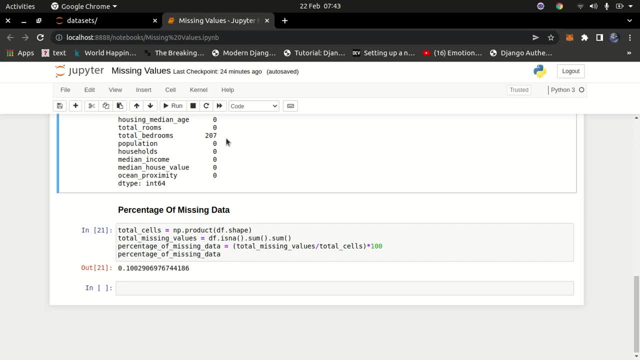 this is not. this is not a large number compared the data set. so if it do not cause a significant reduction in your data, then you can feel free to go ahead and actually drop it. so let me just keep a mark down here. so i just say drop. 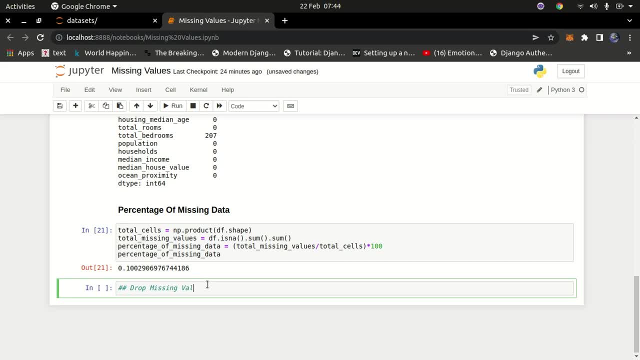 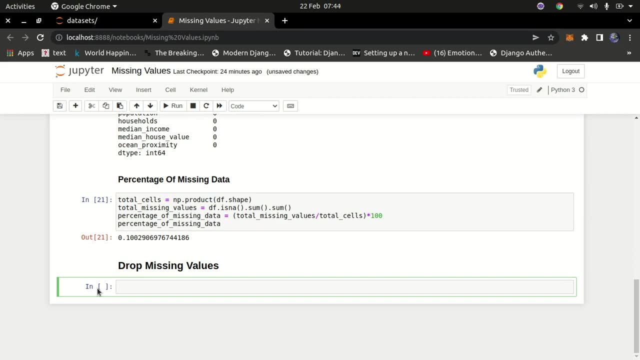 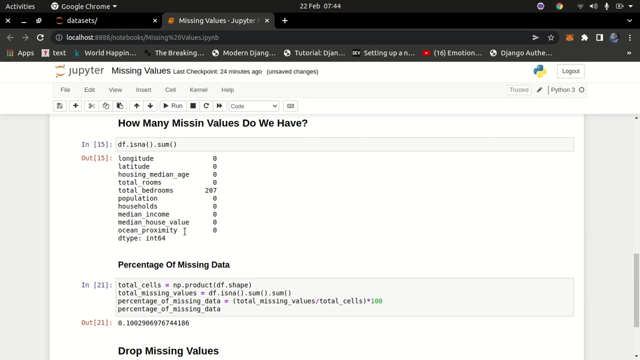 uh, missing, uh, missing uh values. so you want to drop a missing value, in case that the data that is missing is not significantly large. so, in case, uh, in our case here, 200 compared to 20 000 is not not significant, significantly large, so you can feel free to go ahead and actually drop the total. 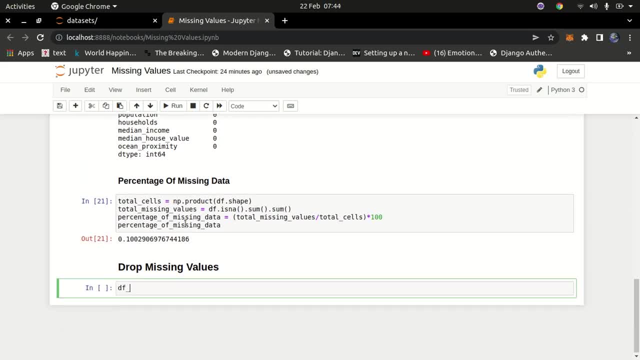 number of bedrooms. so i can simply do, i can do a df underscore copy. i'm going to copy this df. i'm going to df dot copy, copy that data frame. so once i have that data frame copied, all i can simply do i will do df underscore copy: uh dot, drop dot, uh drop na. so 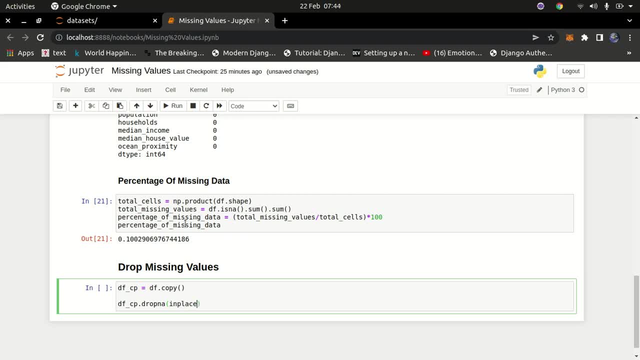 i'm going to drop any values and you're going to say in place. uh equals to uh, true, so in place means that it's going to reassign uh the value back to these specific variables after dropping the columns. so if you don't know about pandas again, you can check out my uh series on pandas. 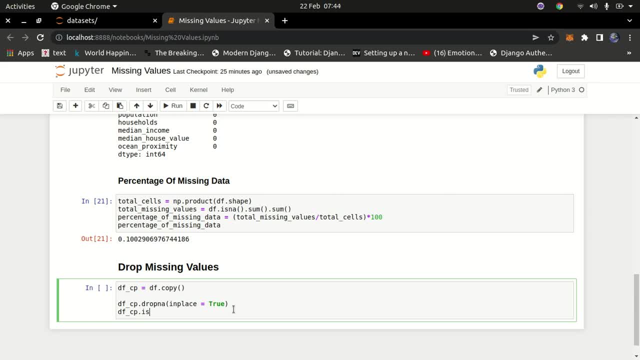 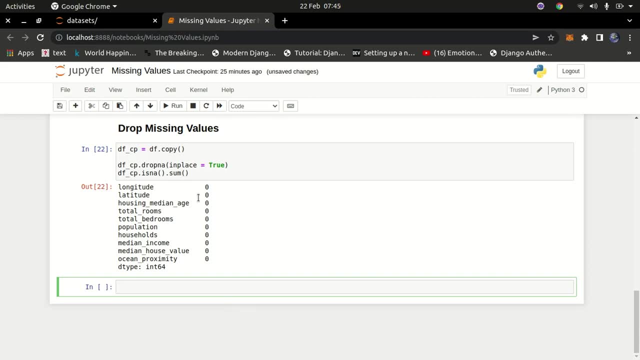 okay, so once i have that, i can do df and the cp dot is n a and then dot sum. okay, check the missing values again. if i do this, we can see i have dropped all the missing values and i don't have any missing values here, so i can also do df and the underscore cp dot. uh, shape, let's. 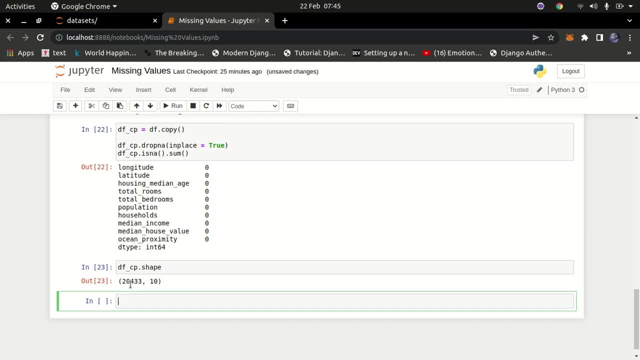 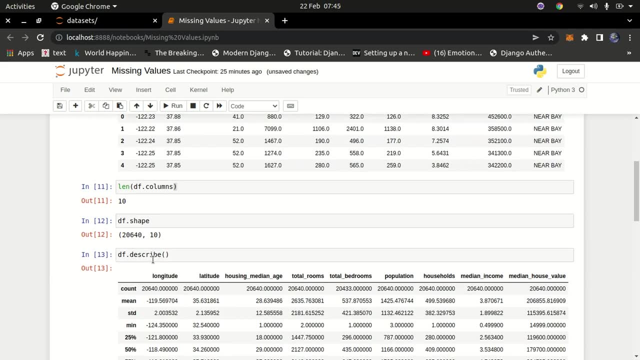 check the value. so you have four, uh, two, twenty thousand, four, four, three, three. so you can check. uh, that is not a a significant drop in the original one, so it was about four, uh, twenty thousand six hundred and something. so it is about two hundred and and seven, right, two hundred, yeah. 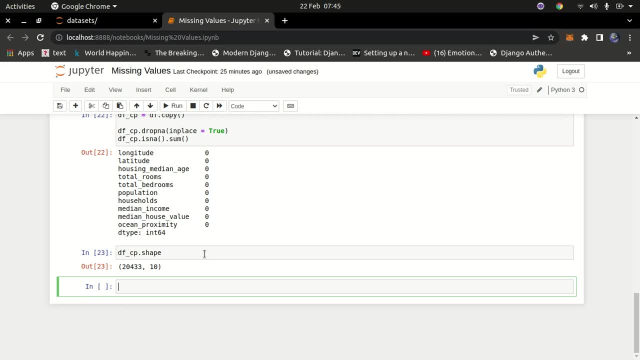 actually twenty and seven, exactly. so twenty and seven uh data, uh rows you have just dropped. so this is not that of a big difference in case in this specific case, but in most cases. in some cases- not most- in some cases this can be a big difference. so, uh, just have. 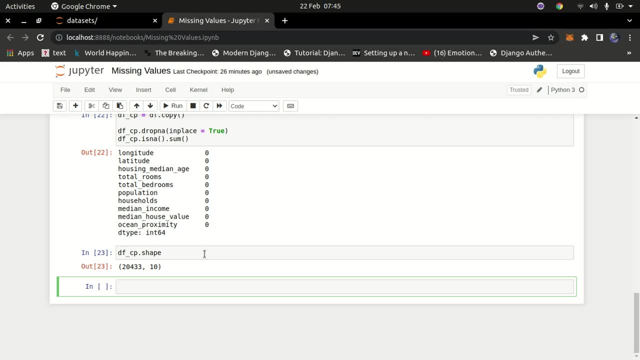 you just have to know, uh, whether, uh, it's going to cause a huge reduction in amount of data. if that's going to be the case, then do not drop it. the other way that you can, uh, deal with the missing values, and let's look at another way that you can deal with the missing file which is filling in the 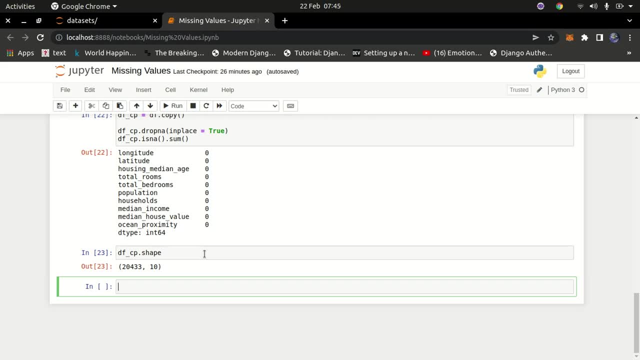 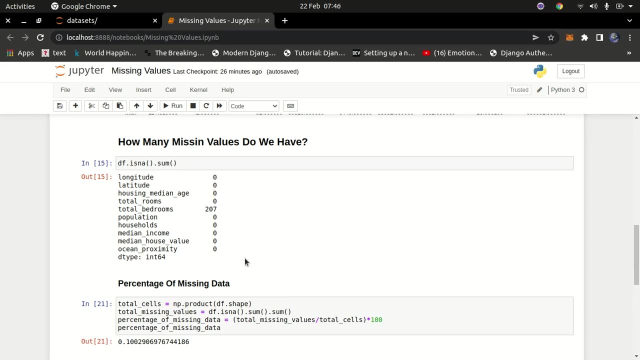 missing values. so if you have missing values, you can actually go ahead and fill in the missing values. let's say that you have the total number of bedrooms. uh, you have done a research and you found that, uh, total number of bedrooms on average is a value of two. so you: 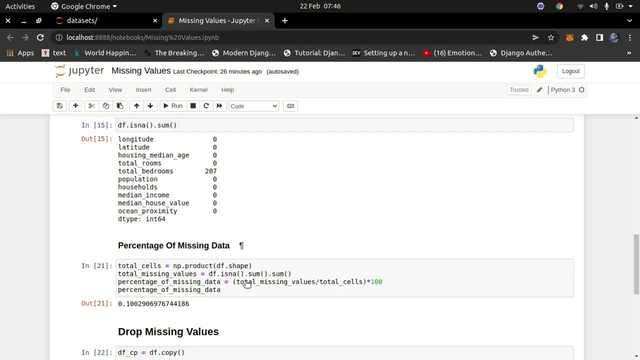 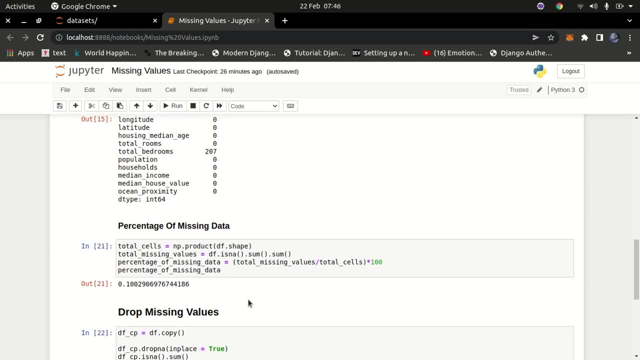 can go, simply go ahead and fill this with the values of two, instead of dropping, so each, uh, each row that does not have a bedroom. total number of bedroom, the number of bedrooms. you can just, uh, simply pass in a two. okay, uh, this and this, uh, if you're filling in a missing values, then you should. 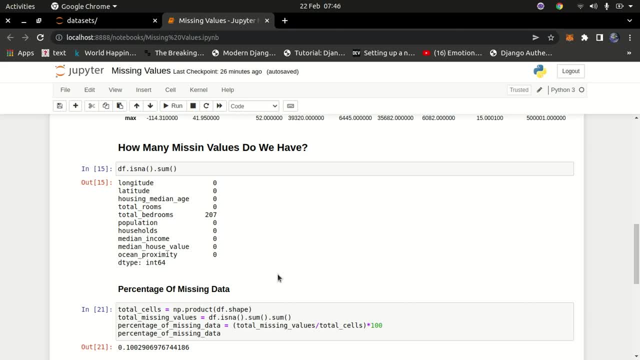 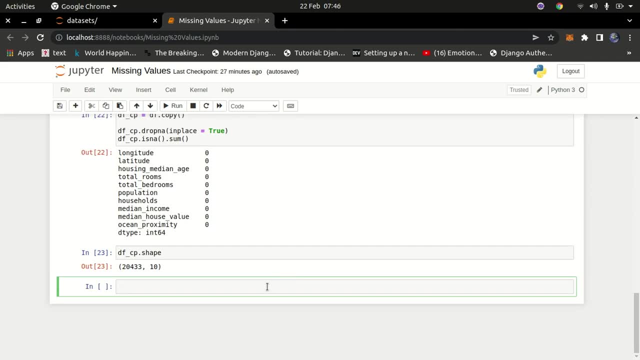 do a lot of research to know that the actual value that you're fitting in is not a bias or it's not fake. okay, so that you have to do research and then, based on that research, that's when you're filling in those values. so let me just keep another mark here in markdown and say: fill in, uh, missing. 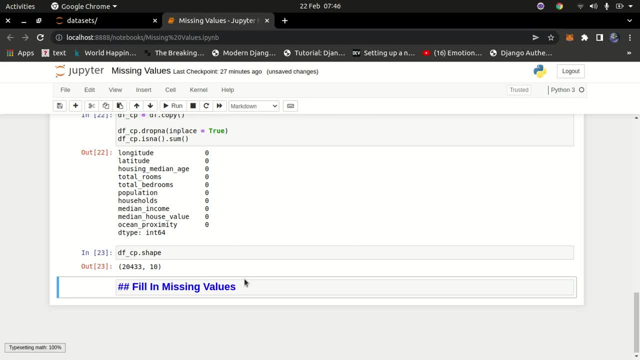 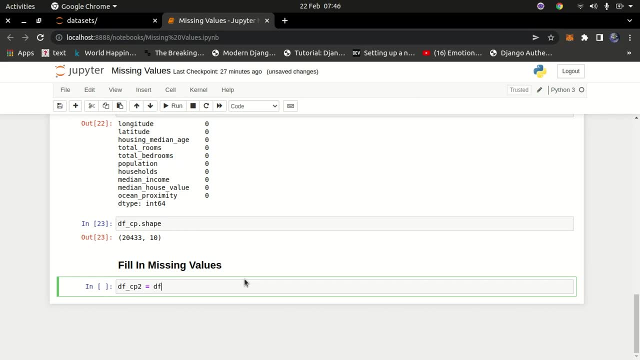 uh, values, just like that, and i'm going to make this to be a markdown cell, so yeah, so once i have that, i can do a df underscore copy and i'm going to call it copy 2, and this is going to be a dfcopy. you're going to copy the original data set and then i'm going to do: uh, simply do. let's check if. 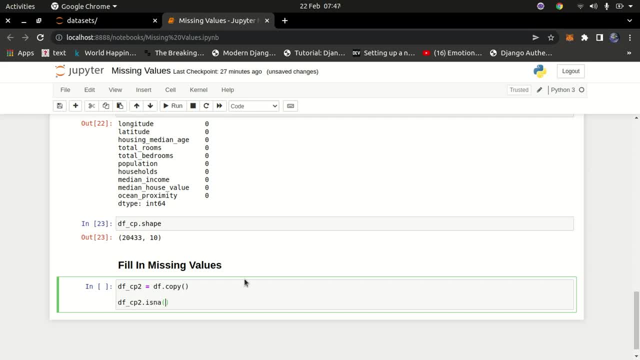 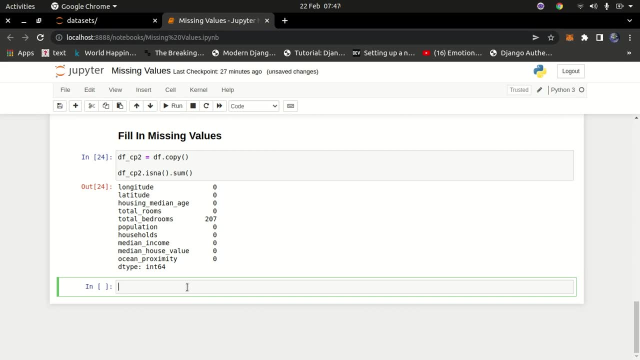 i'm going to dfcopy to dot is and a dot sum and this is going to return to us the missing value. you have two 207 missing values right here, so i'm going to do a df underscore copy to the dot fill and a. so i'm going to fill the missing values. so i'm going to fill the missing values with, simply. 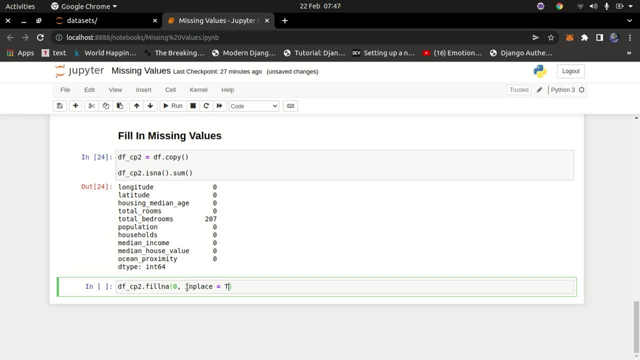 0 and i'm going to say in place equals to true. now it doesn't make sense. i fill the total of bedrooms the value of 0, because by default i think that already you can fill this 0 if you want, but not proper that you can have a bedroom to the number of bedrooms to be zero. so let's say that. 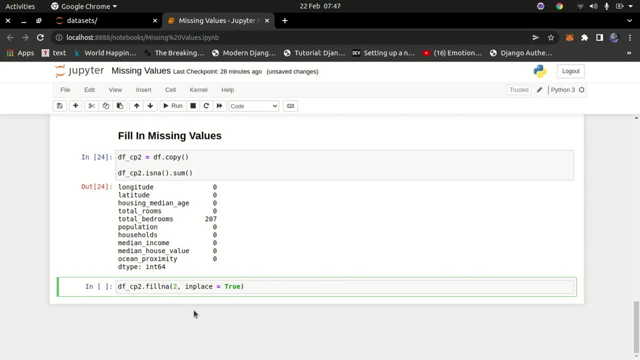 we did a research, intensive research, and we found that on average it can be two. so you fill it with the average value and you just run that. and if you do df, uh underscore, copy two dot uh is an a dot sum. it's going to return to us all of them being zero because we fill all the missing values. 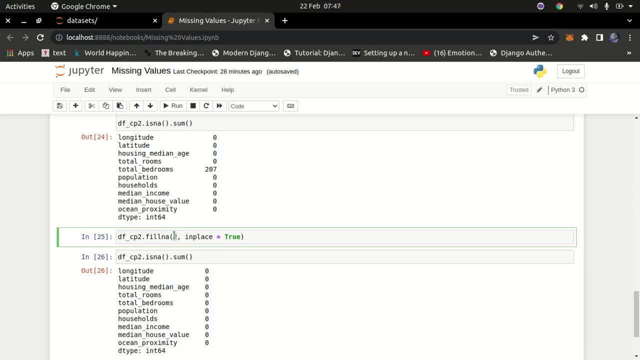 all the missing total of bedrooms, we fill it with a value of two. so this will not only fill this for the the it to fill for all the other columns as well. so if you want to do it a specific, a specific column, then you have to select one in that column. but in this case we have only total. 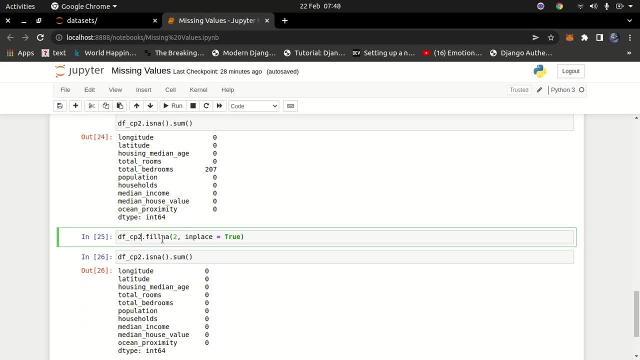 bedrooms missing, so i didn't have. i didn't have to specify it, i just pass into. but in most cases you just have to specify the column itself and then and then fill in that specific column only. so, now that you have looked at how to fill your na values, one thing you also do is that you can. 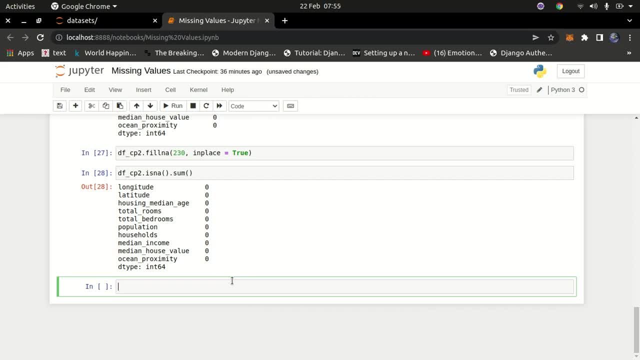 fill in a values with the rows, that with the data from the rows above or below. so in pandas we call this one a forward field or a backward field, backward propagation. so we call this an, an, any an, an an forward field of any backward field. so backward propagation rather. 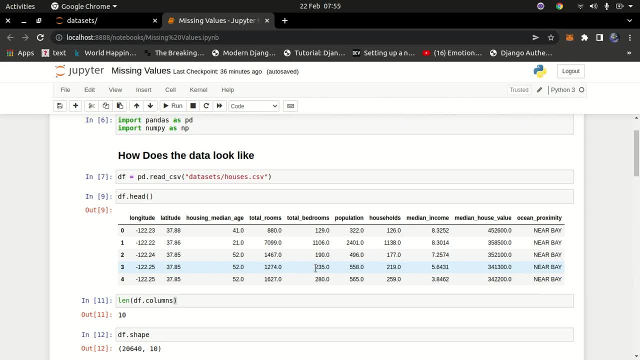 so uh, let me just go in here, for example. let me use this as an example right here. so let's say that we have, uh, we have, uh, we have uh, two five, three missing, right, so let's say we have two five, three missing. one way i can simply solve this is simply: uh, but we're filling this value with 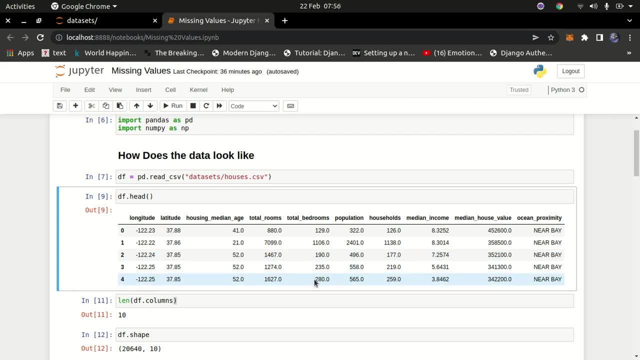 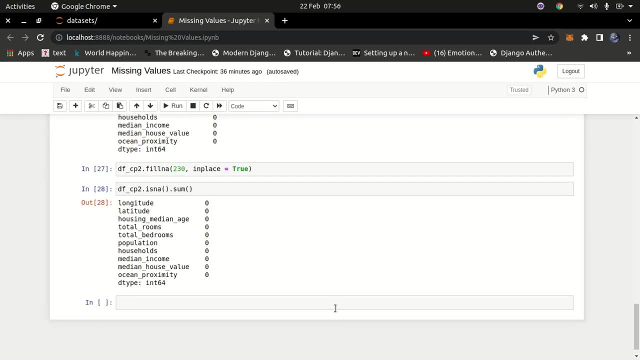 the one that with the row that's above it or filling it with the row that is below it. that is uh, uh n a propagation. you can propagate either backward or a forward, so you can do a research on that. so let me just do a df underscore, cp. underscore three is going to be equals to uh. 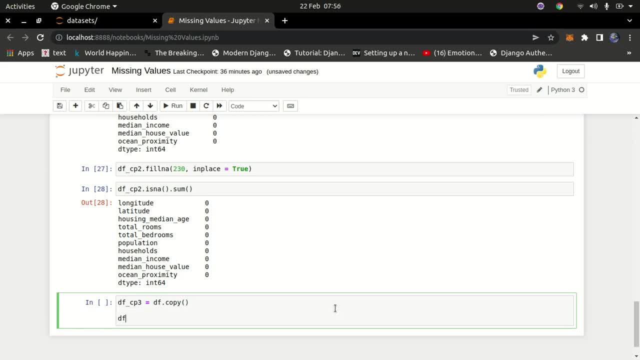 df dot copy, right, i'm going to simply make a copy of it and i'm going to df underscore cp: three dot fill na, and we specify the method, and the method i'm going to use is going to be called. we can do a forward fill, right, so ff fill, or you can also do a backward fill, which is bff me, if you. 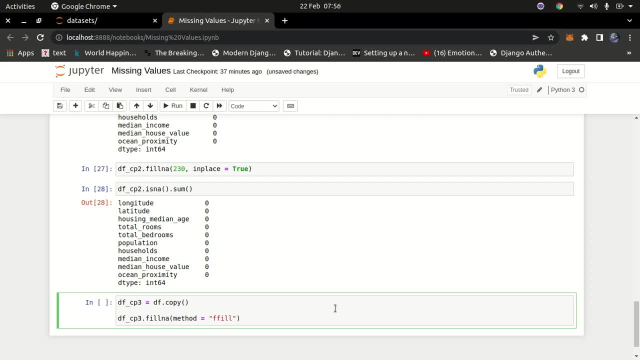 do. a forward fill means we replace each row with a row, each row with a data that is from above it, or it's going to replace each row with a data that is from below it. it's going to be backward fill. okay, so in this case you want a forward fill, and then i'm going to go ahead and specify, uh, the. 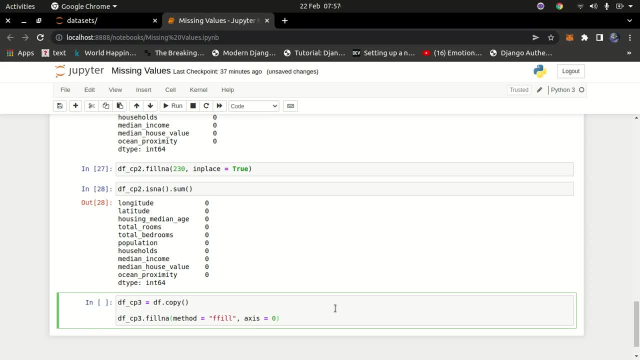 axis, and now i want the axis to be of row, the row axis. so once i have that, i'm going to say uh, in place, and in place is going to simply be true. so once i have that, i can simply run the code and i can also do: uh, df, dot, df. 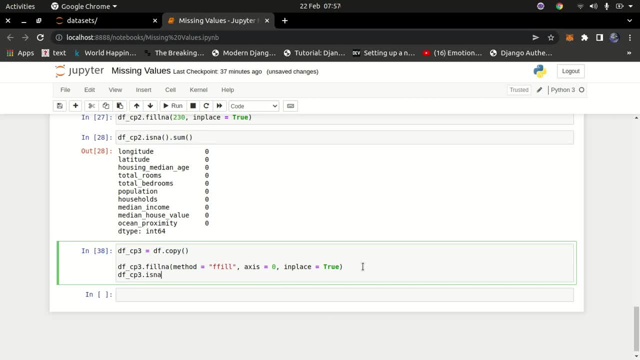 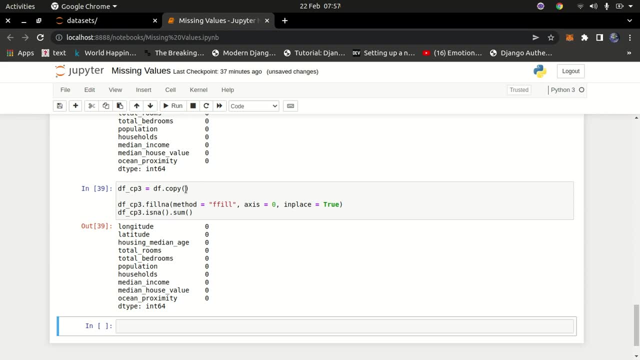 underscore cp3. dot is uh is na dot sum. so if i check this and you can see now i have no missing values in here, but before i was having missing values. yeah, so that's how you can do it. you also do fill this with a backward uh propagation field. so if i run this again now you can see it also. 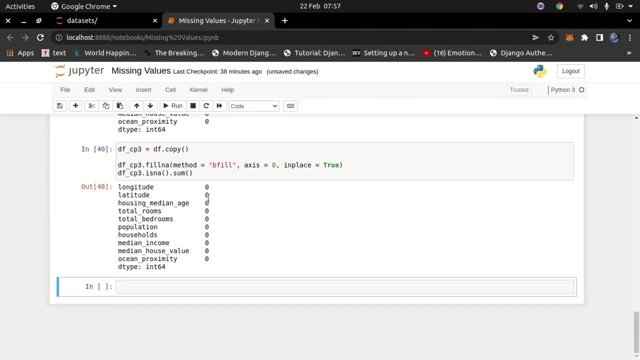 fills it, but it fills with the data from the row below it and not the row before it. okay, so once i have that done, that's- uh, that's one way you can also replace missing values. so, if you work with missing value, this is one way you can- uh, a simple way you can- work with missing. 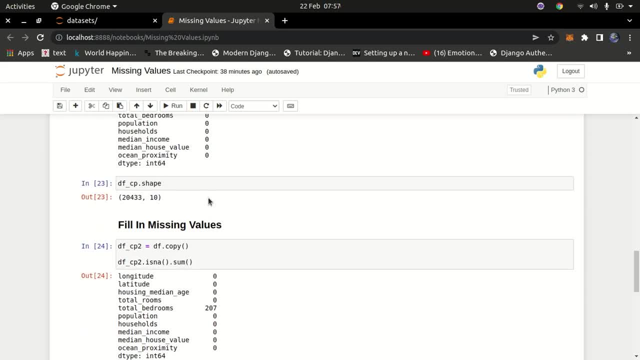 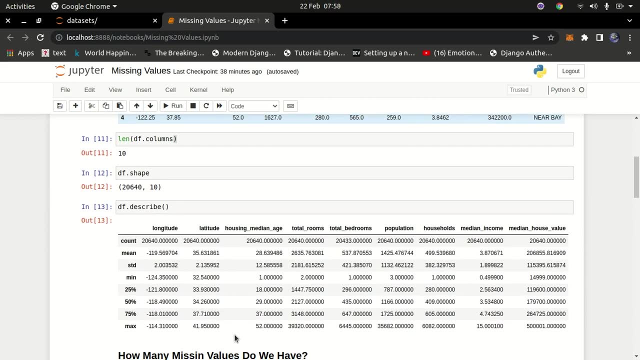 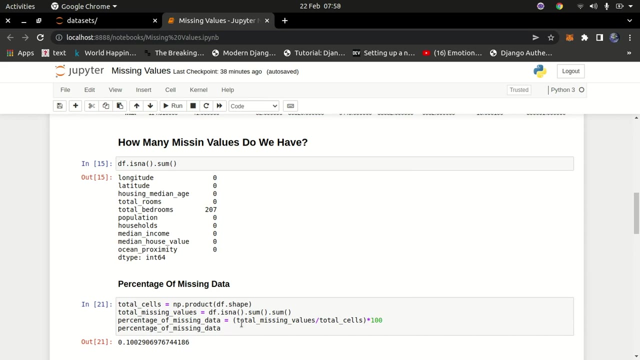 values in uh in one work with panda. so, yeah, that's all i wanted us to cover in this tutorial, which is dealing with missing values. okay, so we went over: uh, how to read a data frame, uh, how to get a look at the data frame to see what data you have and then checking how many uh values do you? 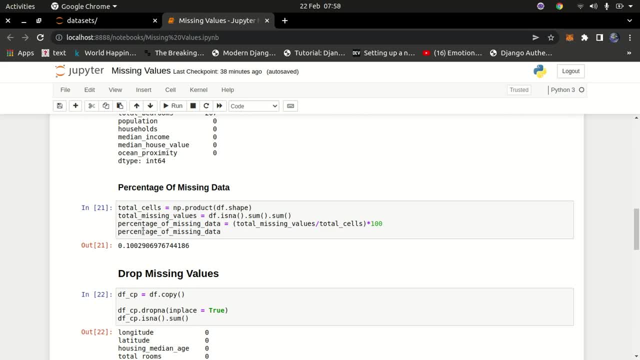 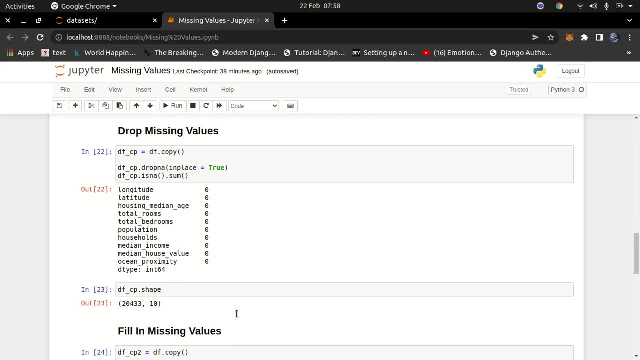 have. how many missing values do you have? okay, and then you calculate the percentage of the missing values and then deciding on which replacement uh method you're supposed to use, whether data is present, it was missing because it wasn't recorded or it doesn't exist, and how you. 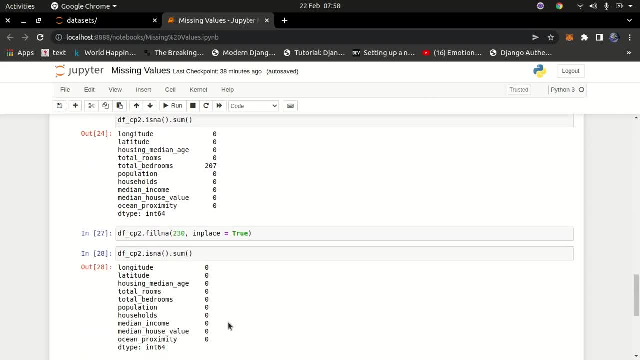 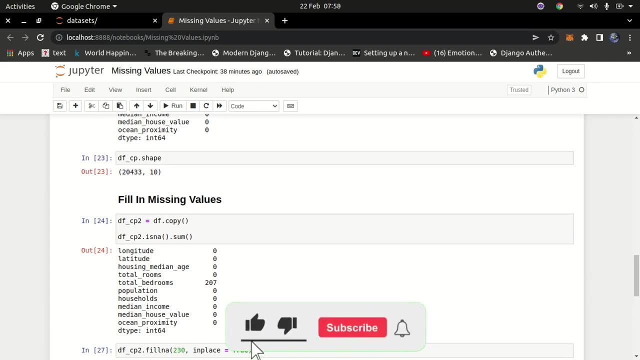 can go about doing your research and feeling those specific values. so, yeah, that's all we're going to cover in this tutorial. so if you're into this tutorial, so far, give this video a thumbs up and subscribe the youtube channel and share this video with anyone who you. 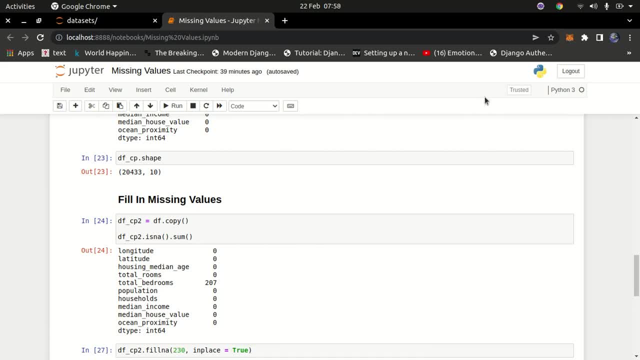 think might find this helpful. so thanks for watching and see you in the next one. keep safe. 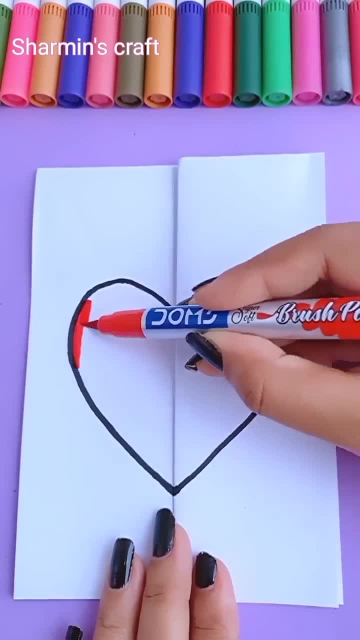 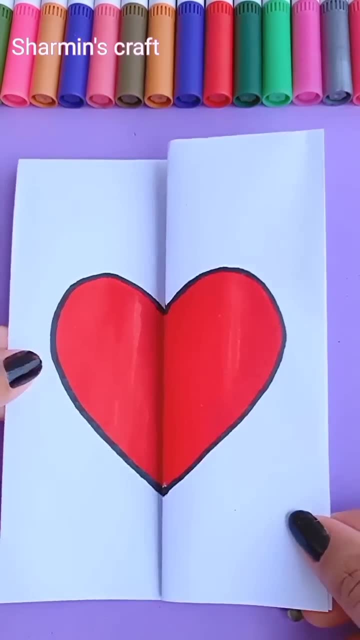 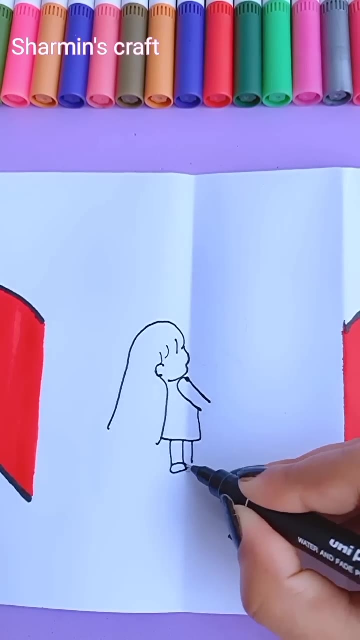 I know you told your friend you're not okay And tell me what's wrong and why you never said you felt that way. Guess you're trying to stay strong and fake a smile until I look away, But I've known you too long. it hurts to watch your blue eyes fade to gray. 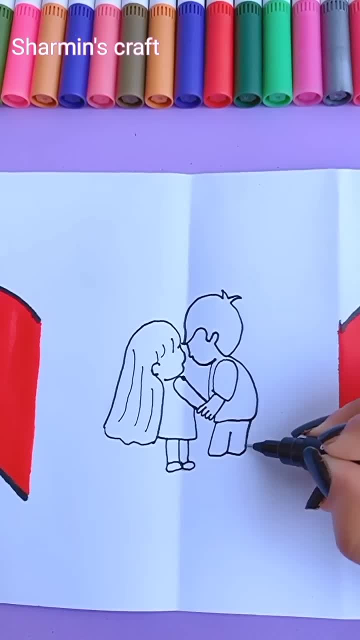 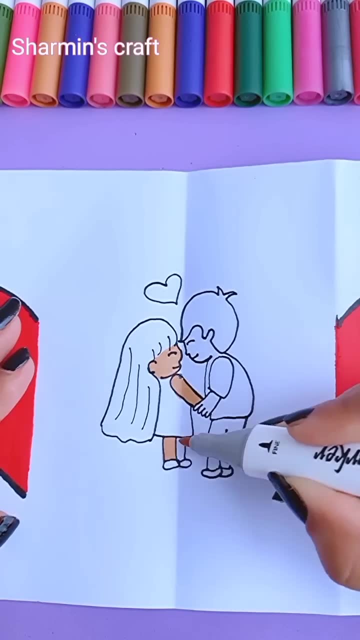 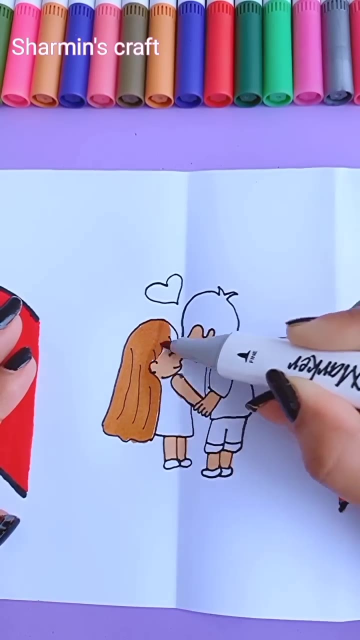 As you fade away, As you fade away. Yeah, I'm about to fade away, Cause every time I wake up I feel like it's Monday. Something's going wrong with all the chemicals up in my brain. All of a sudden, I don't look at anything the same way. 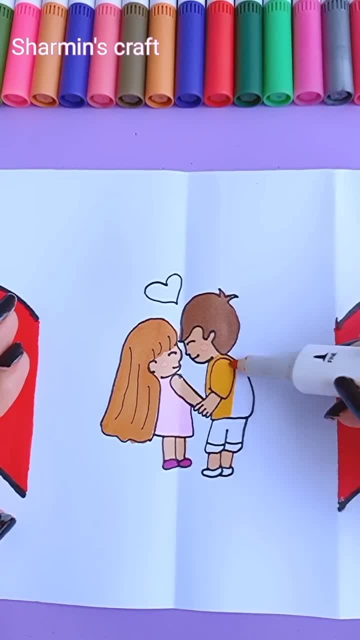 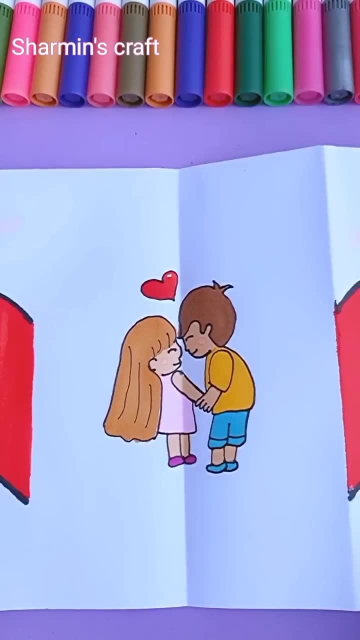 Gotta build up all my thoughts sitting in an ashtray. I'm sorry that I'm so inconvenient. okay, Just let me be me and I'll stay out of your way. I can see the way you look at me. I'm such a disgrace. 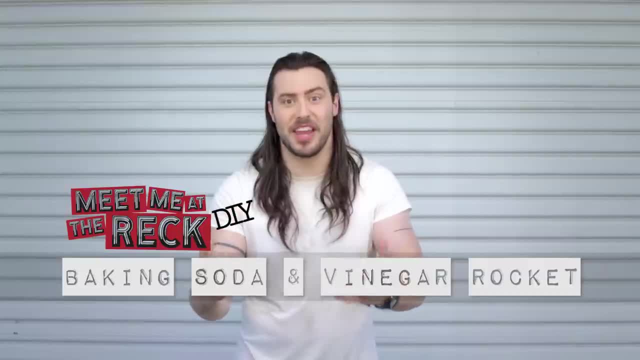 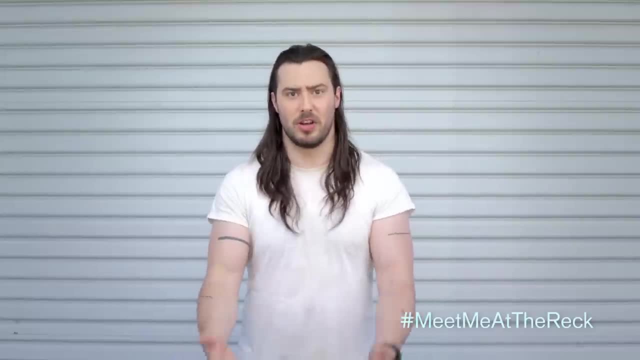 Wreckers. the most fun thing to do in the world is to shoot something up into the air, Am I right? Well, watch us launch rockets in the Meet Me at the Wreck episode called Let There Be Rocket. Want to know how to do it yourself? Well, of course you do. Let's rocket.